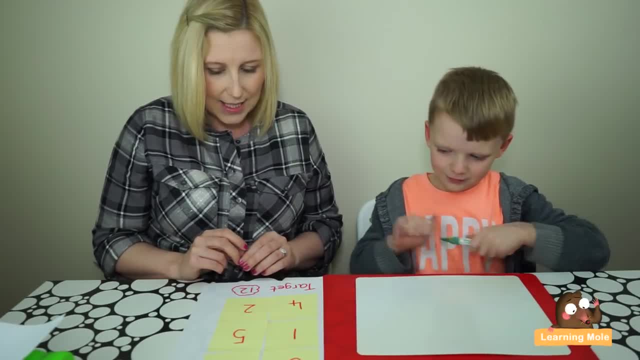 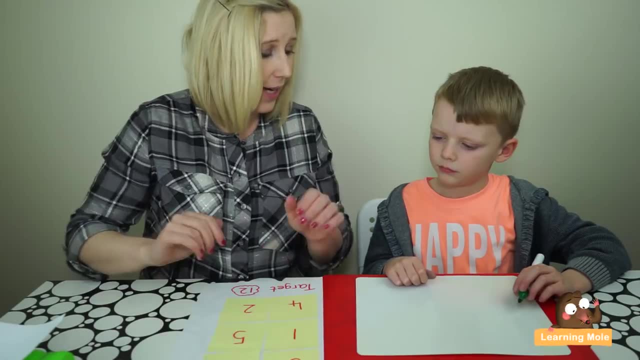 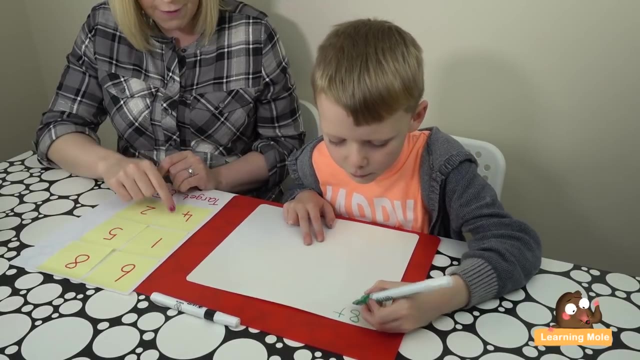 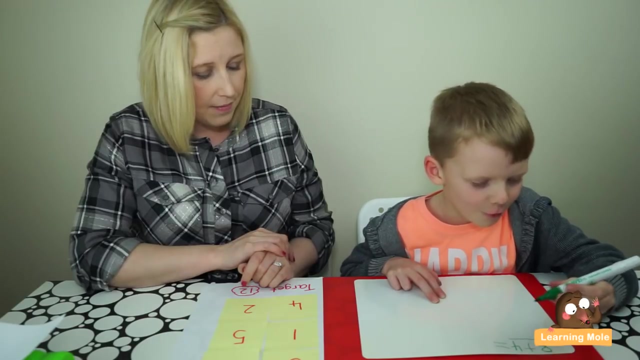 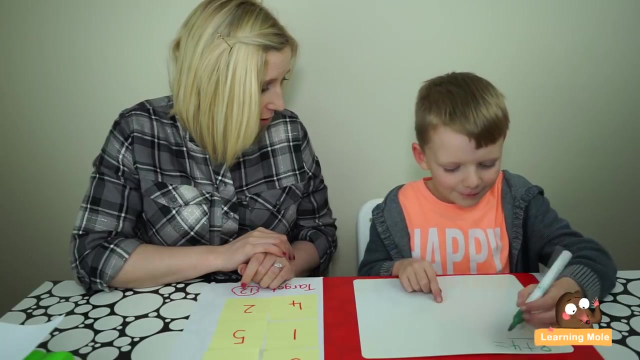 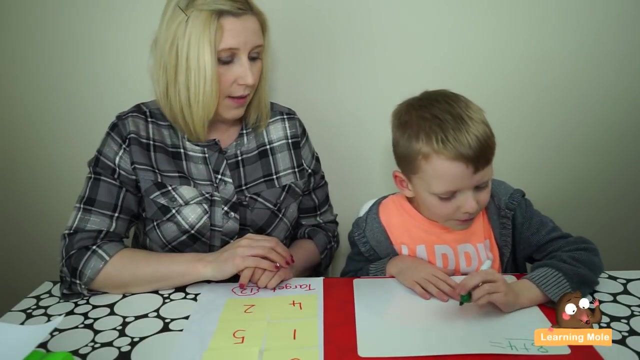 yourself, okay. So let's see, I am going to say I'm going to choose eight, or you can write eight down. okay, eight plus four equals what? Eight plus four equals what Twelve. Good boy, How do you do that? You saw it in your hand, did you Okay? Okay, I'm going to ask you: could you show me how you did? 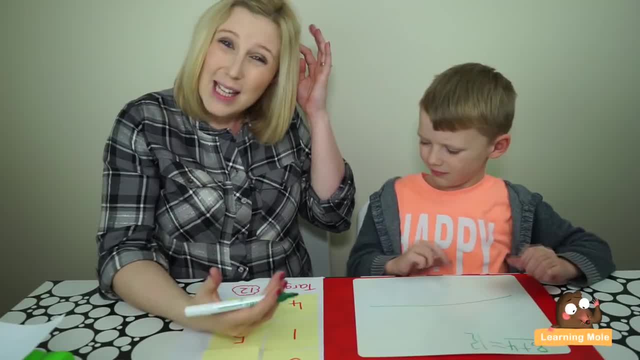 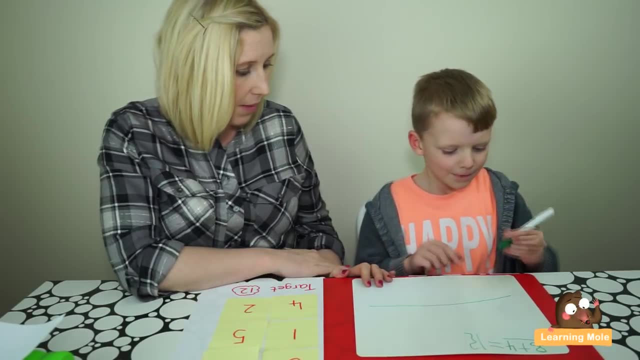 that on a number line. So here's a blank number line. So again, getting your child to explore different methods as well, just to really make sure that they are having that good understanding. So here's a blank number line. What number is going to go at the beginning? One? No, don't need numbers. 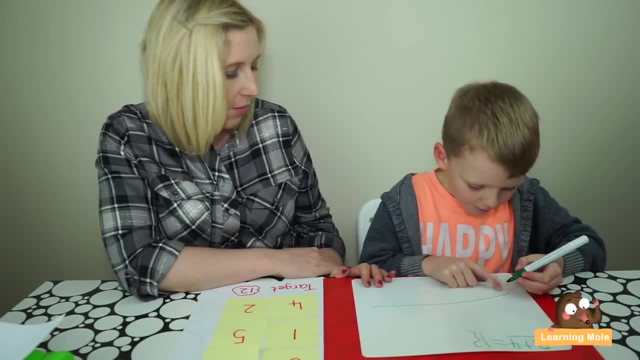 on it. it's a blank one, Isn't that a clever one? You can put one in there. So here's a blank number, and you can put whatever number you want on it. So what number are you going to put at the beginning? 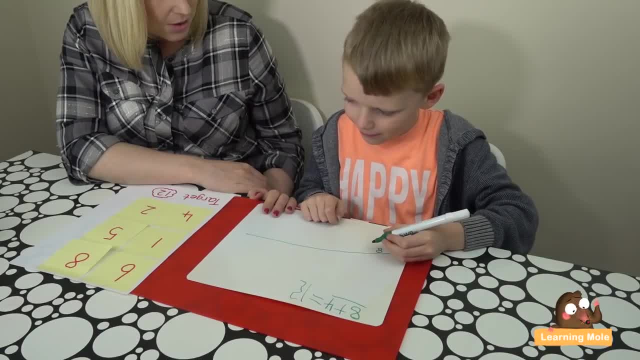 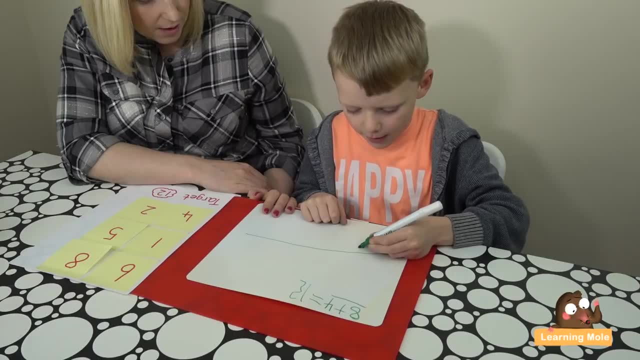 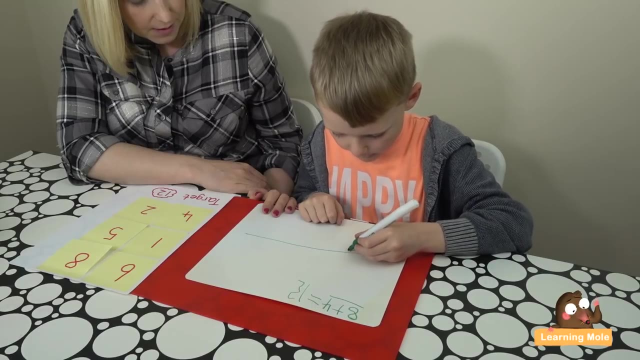 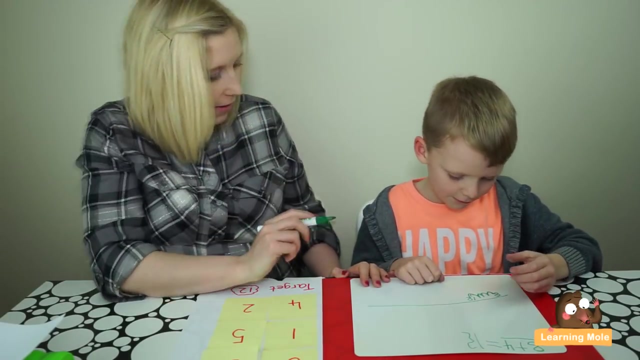 Eight, Yeah, and then how many jumps are you going to do? One, two, three, four, And what number are you going to land on? Twelve, Good boy, Let's just check. Eight, nine, ten, eleven, twelve, Good job. 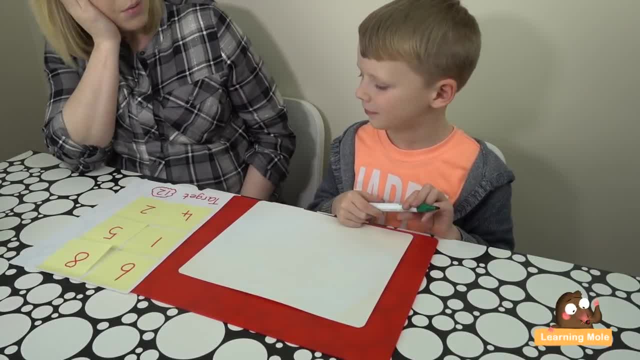 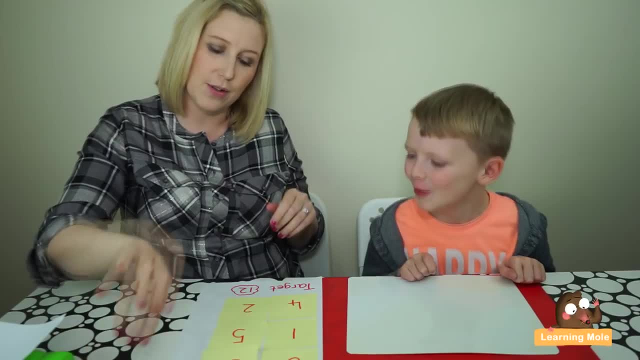 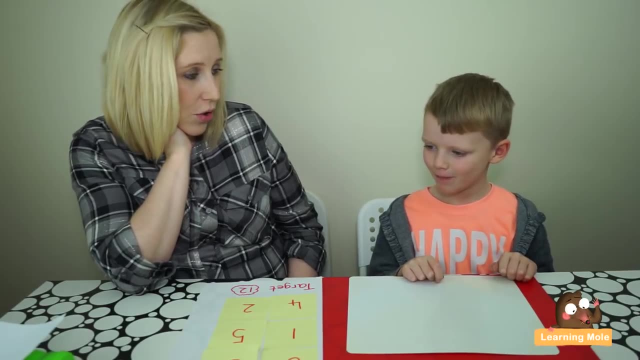 Do you think You can make twelve? So you can take the post-its off if you want, okay. So you might need one number, or two numbers, or three numbers, or you might need to do some adding and you might need to do some taking away as well. So let's see. So choose two numbers to begin with. So this is a really 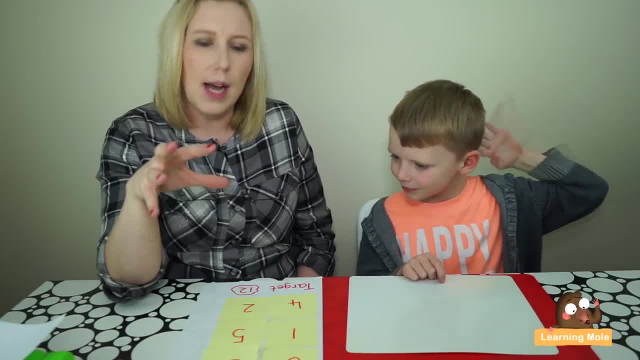 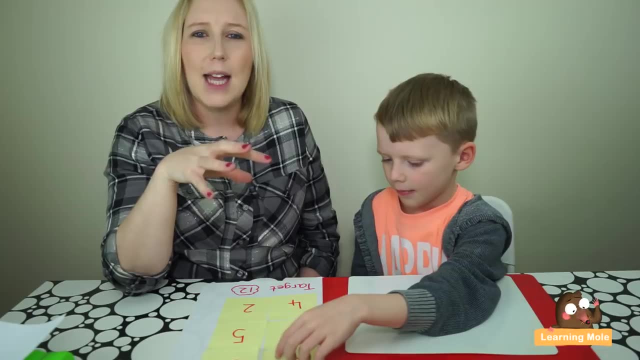 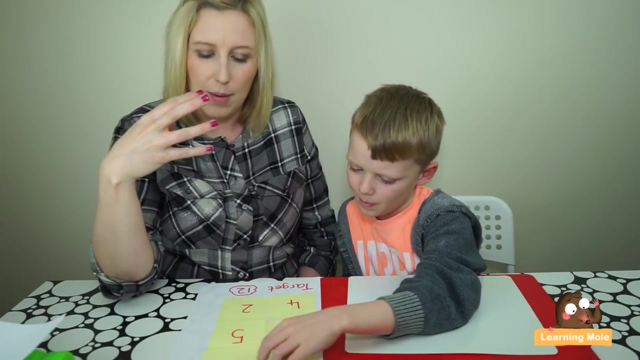 challenging activity. I wouldn't start this activity with a child that's still focusing on adding and taking away, but Aaron is a wee bit more advanced than that And he really likes the idea of a challenge and he sees those connections between numbers. So this is one where you want to push your child and progress him a wee bit further. So what are? 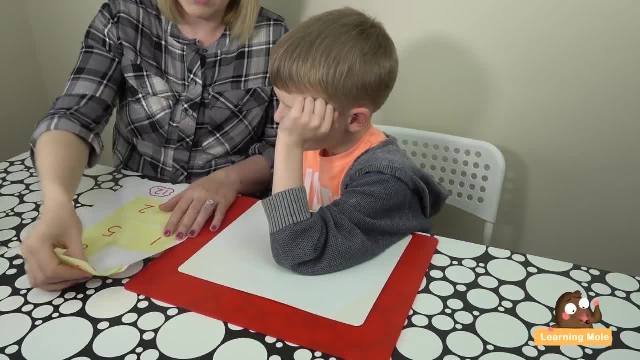 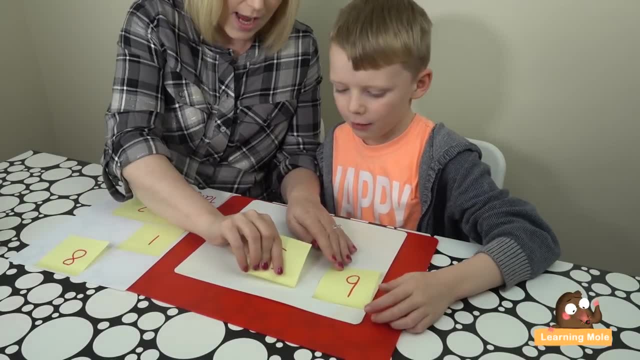 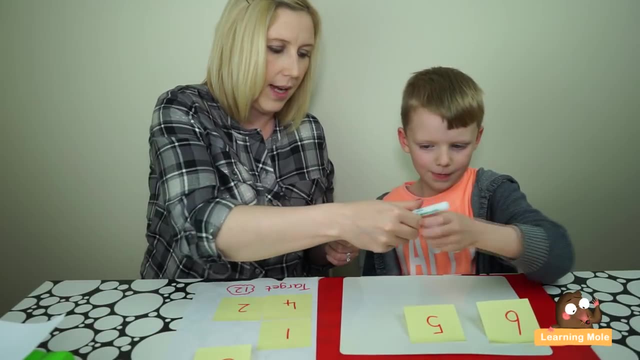 you going to choose Six and five, Right, six and five, okay. So what are you going to do with these? Are you going to add them? Are you going to take them away or what Add? Right, okay. So put your adding symbol in there Six plus. Put your adding in there Five. 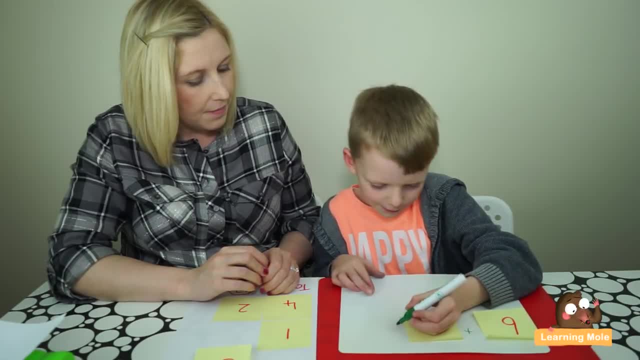 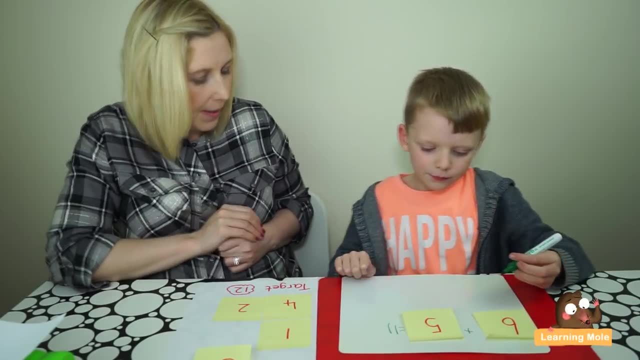 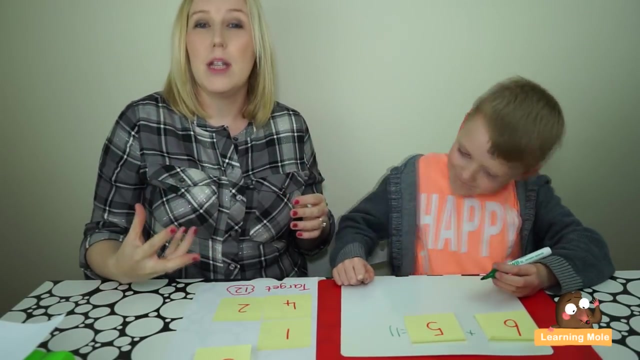 Equals what? Seven? I should know this. Okay, so equals eleven. So have we got to our target number? What is our target number? No, No. So this is where you're really challenging your child. You're pushing them to think a wee. 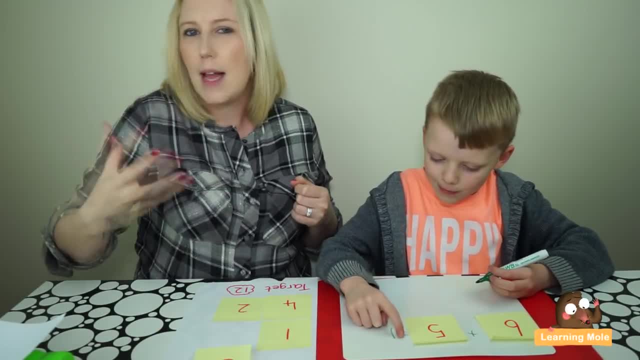 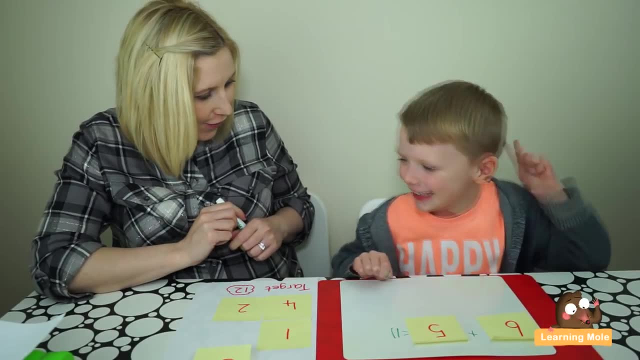 bit more outside the box, You're getting them to think that wee step further. Okay, so, Nunu, that's right. Is there anything else we can add? to make it What? Make it to twelve One? Yeah, we could add one as well. So do you think we could have three numbers in our calculation? 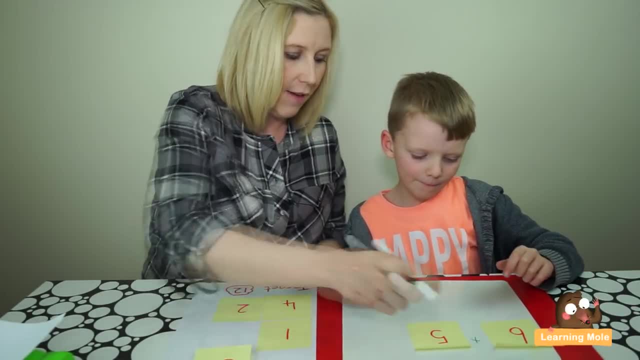 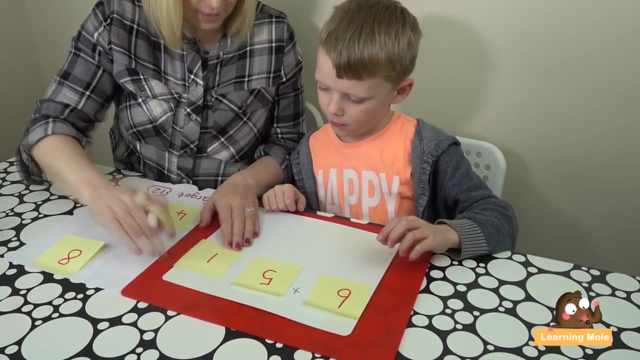 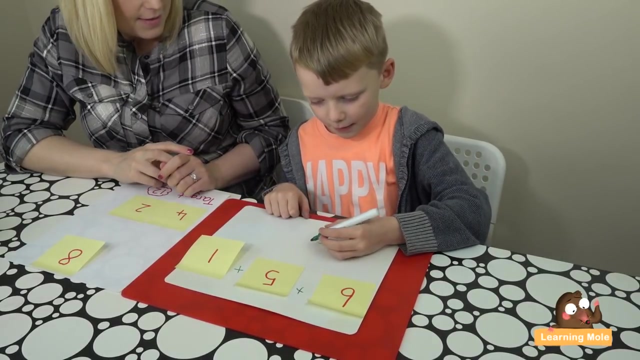 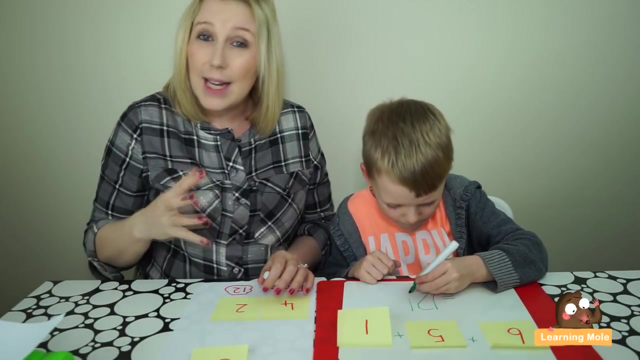 Yeah. So let's rub that out and let's have six plus five plus one. Now try and work it out, and what do you get? Sorry, I'm stealing your pen on you. So now we're getting them to that idea of the concept of adding three numbers, and we're going to even push him this a little bit harder. 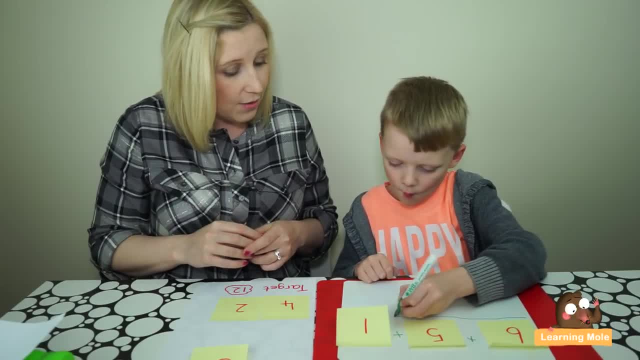 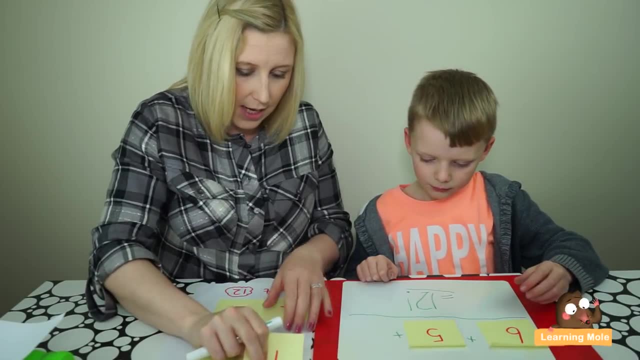 and really get thinking about those relationships. So good boy. So you've got six plus five plus one. Okay, right, Ready, Put these back on the board, Okay, and you're going to try different ones now and see if you can get to twelve again, right? So what are you going to choose this time? So, just by, 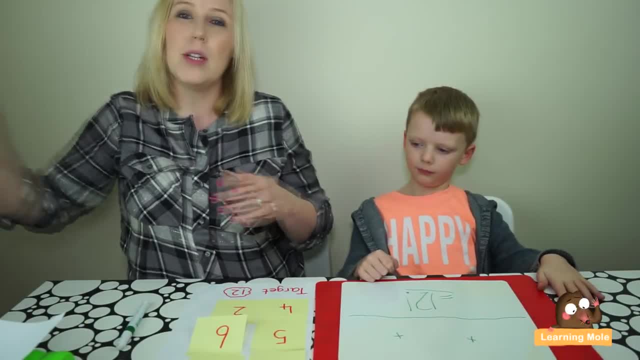 letting them choose those initial first numbers. it gives them the opportunity to think about what they're going to work with and how they're going to develop their relationship with the child And how they're going to develop that and how they're going to push themselves that way a bit. 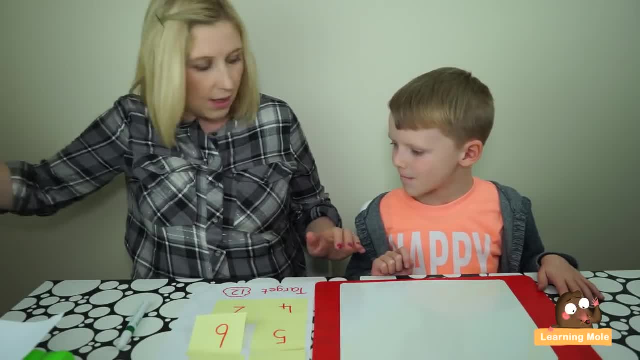 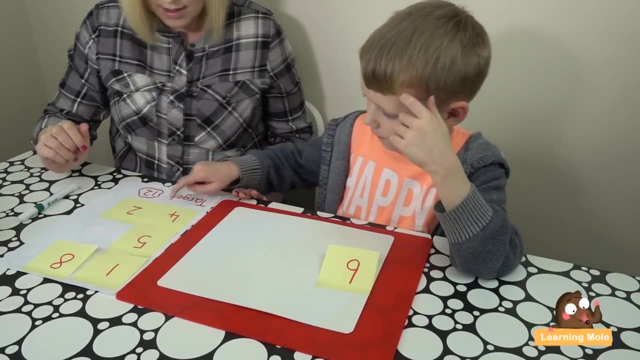 further. You should have kept the twelve. Yeah, well, we might not have room, Okay, so what are you going to choose? again, Six, this time again. Six, Six, Four and two. Okay, six. Are you adding or taking away? What are you doing? 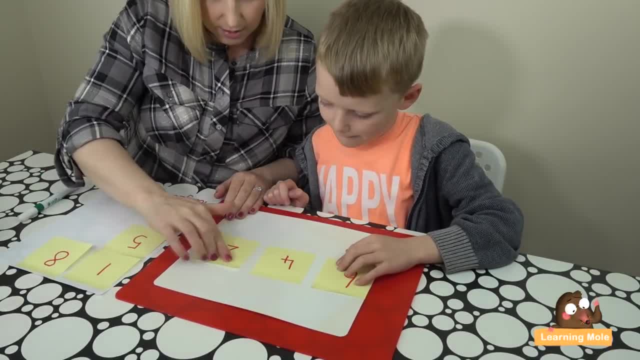 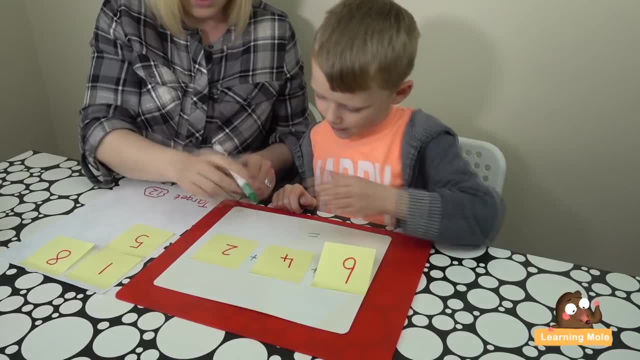 Adding again. You're going to add them all. Yeah, Okay, right, Actually, what I like, Let's see. Let's see Six plus four plus two Equals. You work it out for me. So immediately he's went for that idea of adding those three numbers again. so he's taking on what? 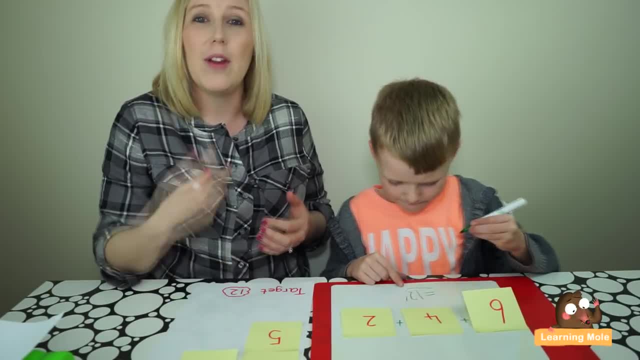 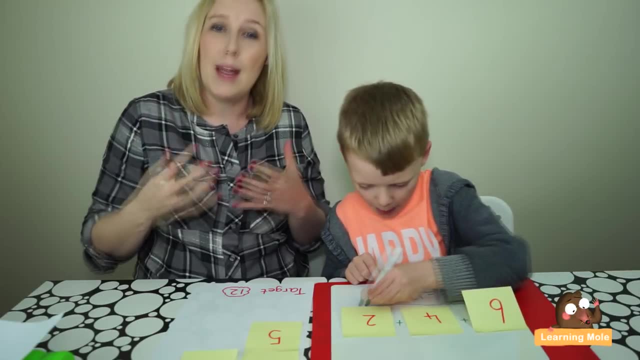 on board what he has learned and he's pushing himself that little bit further. and that's what we want: to encourage and push your child so that they are making that progress, making those connections and putting that maths into context. How did you know it was twelve? 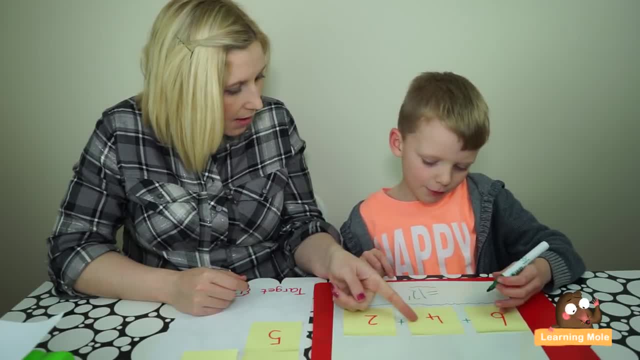 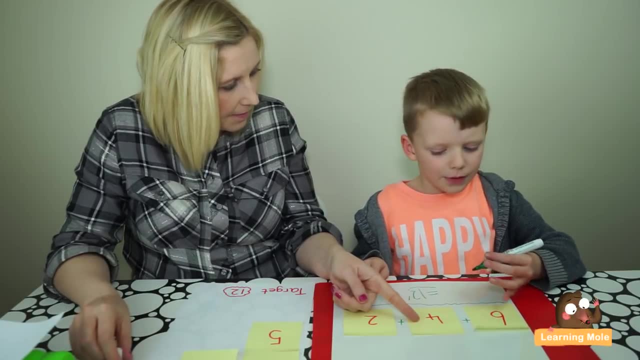 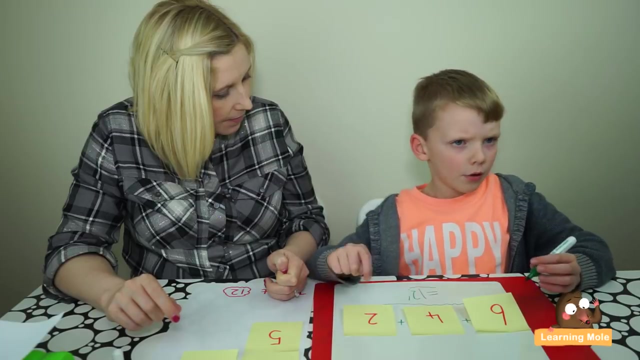 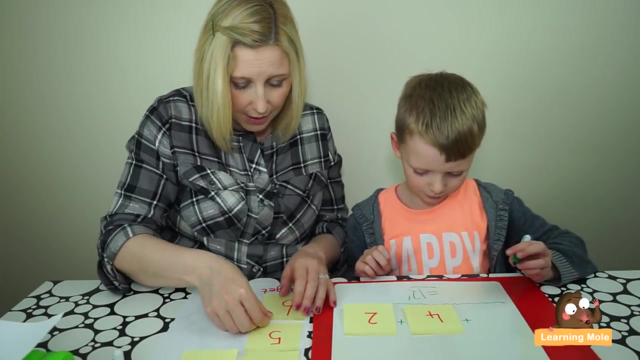 Well, six plus four, Well, you know, you know that That's ten. Oh, and then you're going to add your two on And ten, And ten plus two is, you should know, is twelve. Good boy, Well done. So we found another way, So let's stick these back on again. 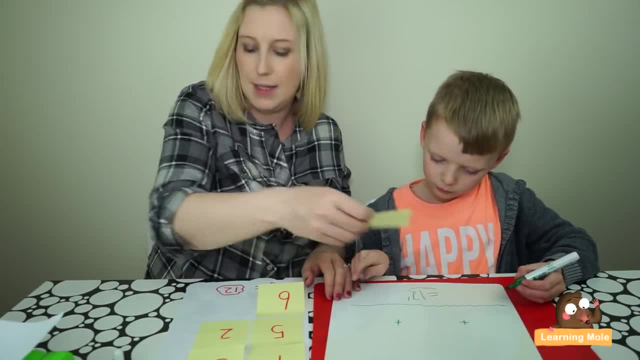 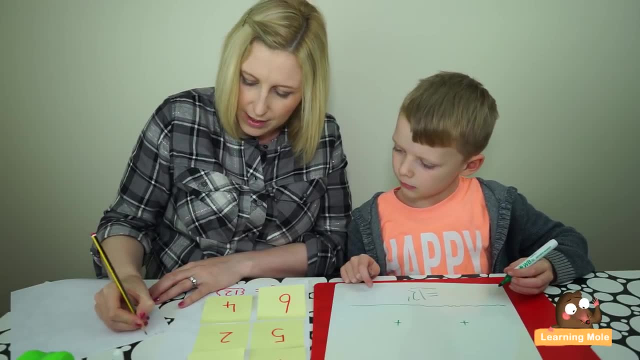 and do you know what I'm going to do for you, Aaron? On this blank piece of paper over here, I'm going to write these all down, so we don't mix them up. So what do we have? We had eight plus four plus twelve plus four- Yes, it was twelve, and we had 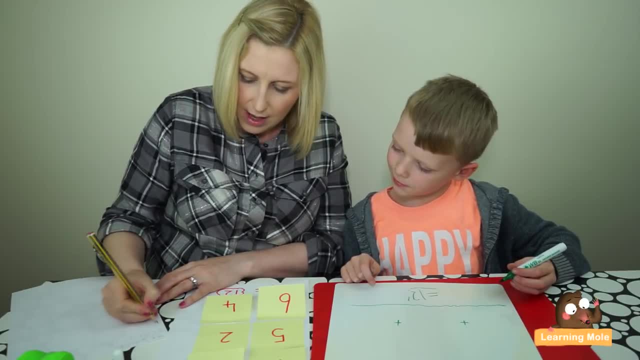 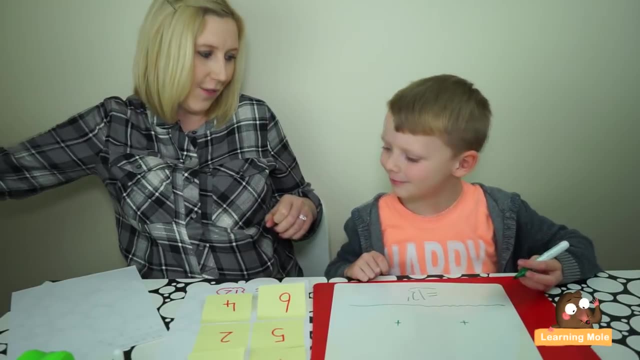 Six plus five plus one, which was twelve, and we had six plus four plus two. Now I'm going to really challenge you this time. This is going to be even more difficult. Do you think you can do it? This time, I'm going to ask you to see if you could do a taking away. 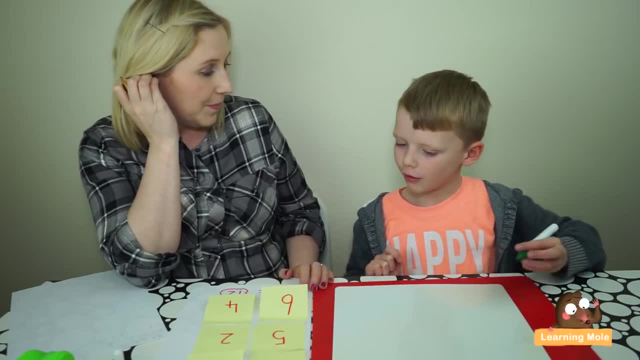 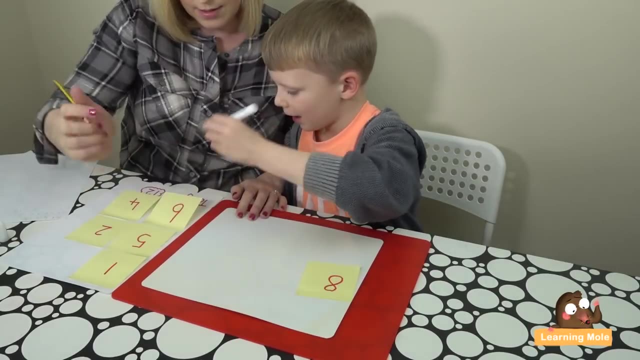 But you might need to do some adding first. So let's see what are you going to choose now. The biggest number, eight, Okay, and what are you going to add it to? I'm six Right. eight plus six Right. we'll do that bit first and see where we need to go. 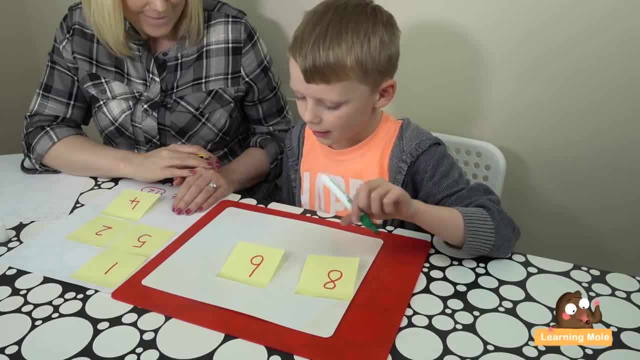 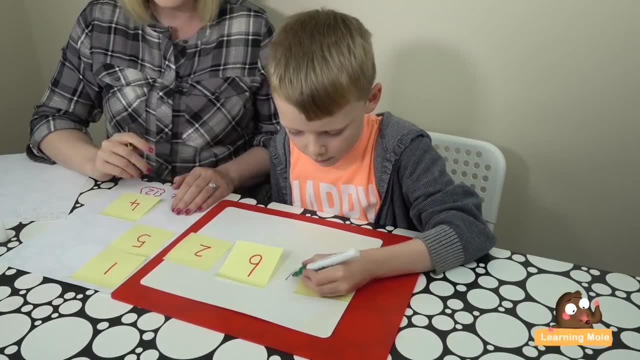 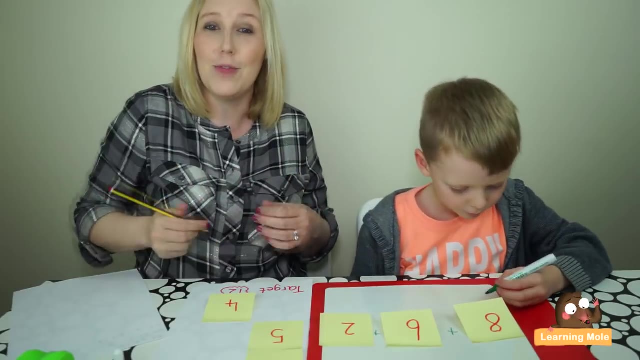 And take away. Take away two. You think it's going to be. take away two, Right. write out your calculation, then Put your symbols in. So immediately he's starting to think about what he needs to do to get to that target number, and this is where we really want to focus. 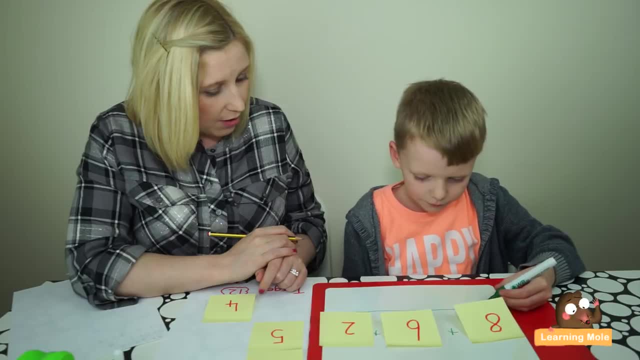 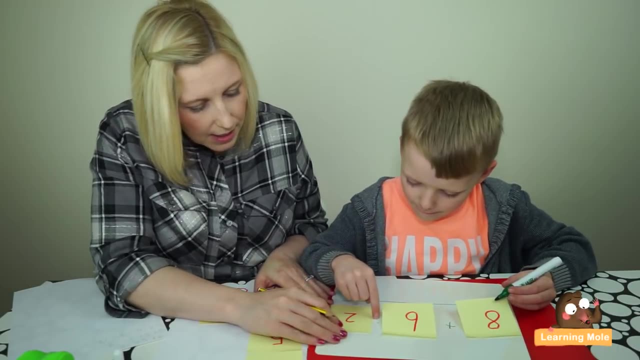 Okay, so let's check. So what bit are you doing first, Now you've done a plus in here. Should that be a plus? No, What should that be? Take away, That should be take away. Okay, so put take away in there. 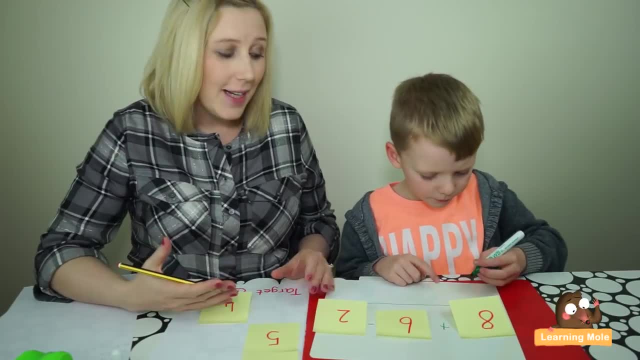 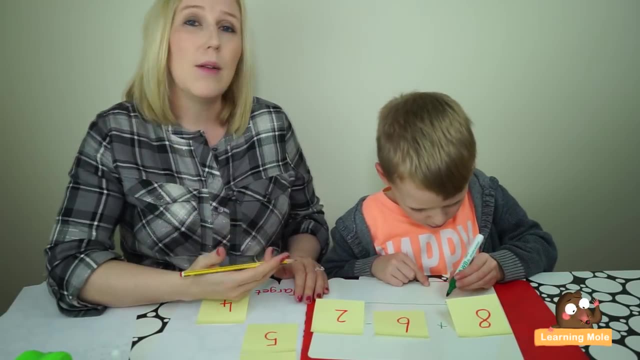 Right now. tell me what you're going to do first. So Aaron has decided he wants to use a number line, and that is great. Encourage your child to use whatever method they feel most comfortable with. So he is working on his number line to add his six and his eight. Okay, good boy, Well done. 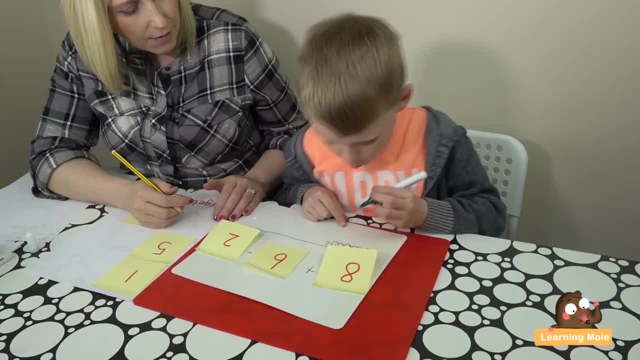 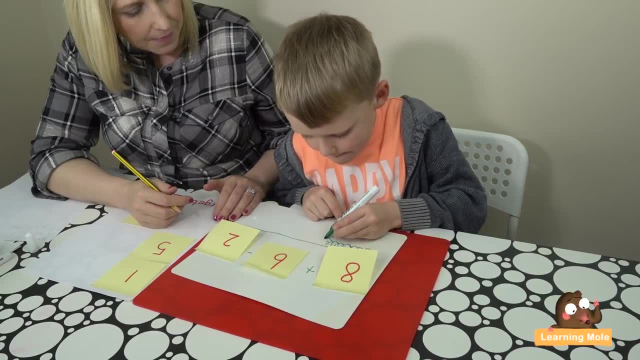 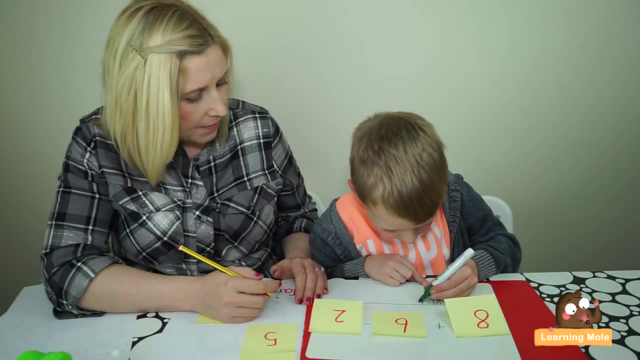 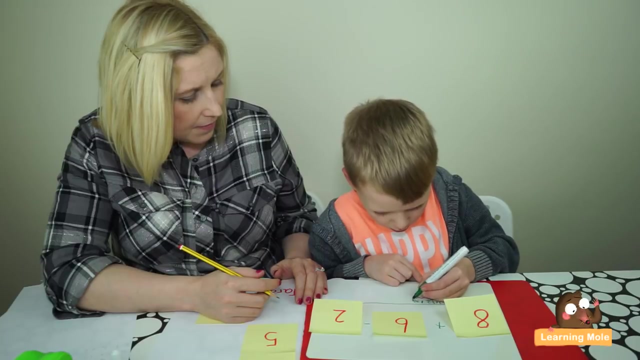 How are you going to know how many jumps you've done? Have you been checking? I've been checking recently. Okay, so you're not there. You're not there because you have the biglective. That's not a big light weight. 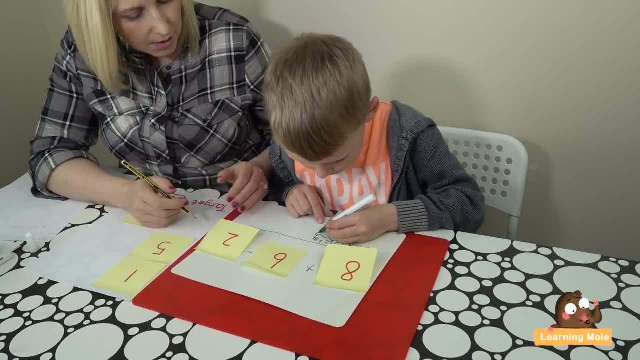 Okay, So okay, I'll give you an example. I'll give you an example. Okay, so Okay, I'll give you an example. I'll give you an example. So you have a good answer, She'snow, if you want to put that, you know that it's gonna help you a little bit. 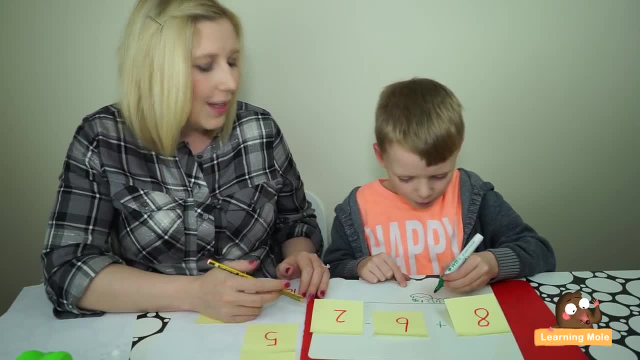 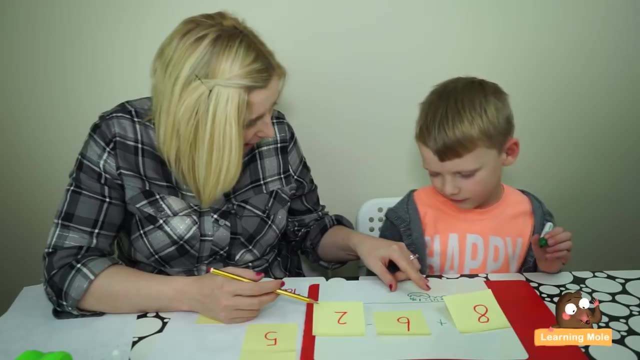 Okay, Yeah, You don't have to wait. and three, oh, i understand. then you're going to go back and then go back two. so you've done six plus eight gets you to 14, and then you've went back two to get you to 12. good boy, excellent i. 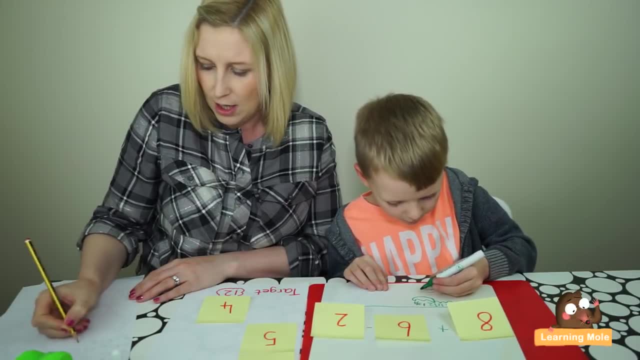 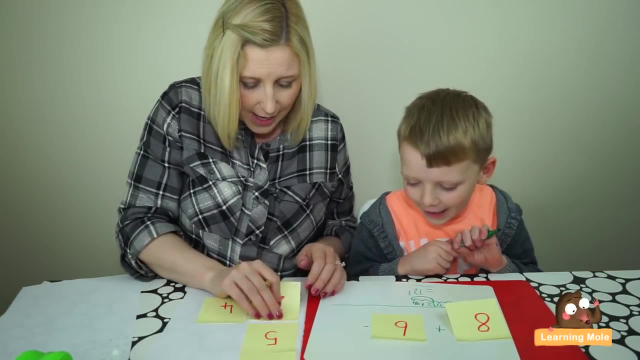 love how you've shown that on your number line. that is really really good. okay, right, excellent. so do you think we could do one last one with the taking away? you're really and pretty, really impressed me with this, siren, because this is really difficult, but you've really really been. 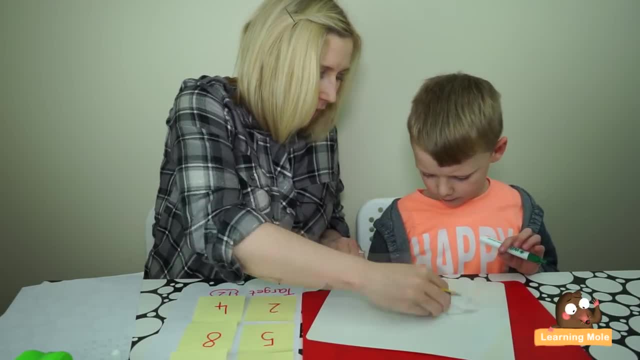 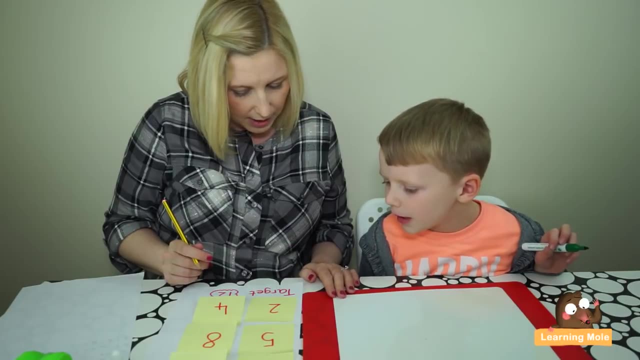 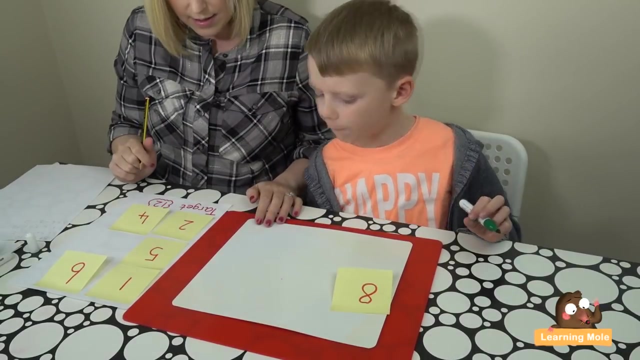 thinking sensibly: right, okay, right, so see if you can do another one that begins with adding and then ends with taking away. well, what do you think you're going to start with? eight again, okay, and five, okay, and what are you going to do to eight and five? 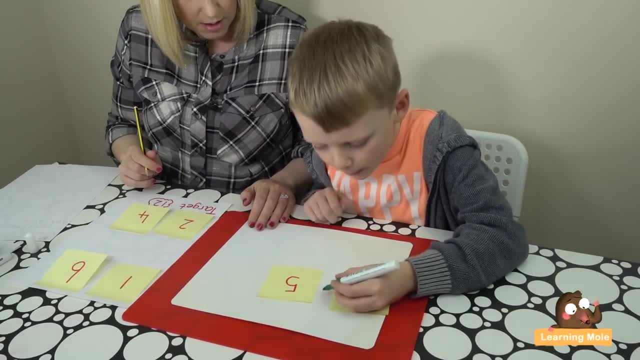 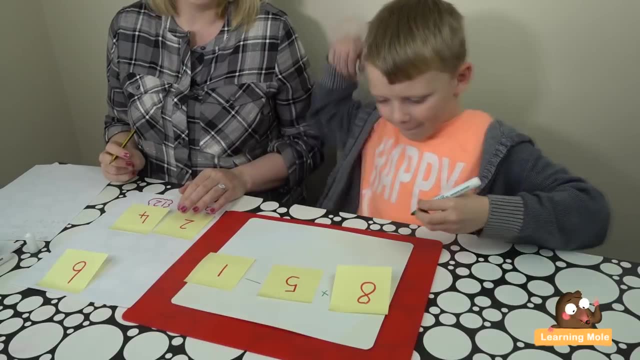 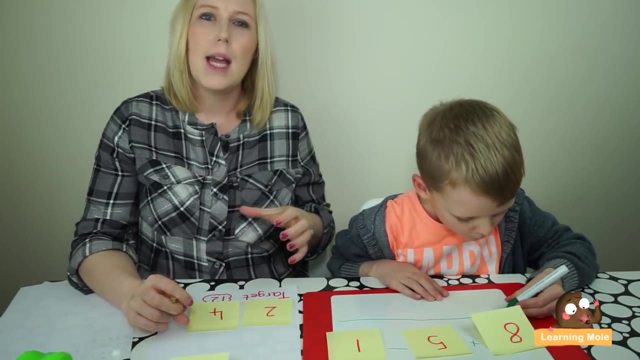 take away one. take away one, take away one. okay, right, let's see if you're right, right, you can do your working out. so it's great to see that aaron has is choosing the numbers. he's thinking about the symbols, he's thinking about the relationship of getting the number bigger and then coming back again on himself, and then he's. 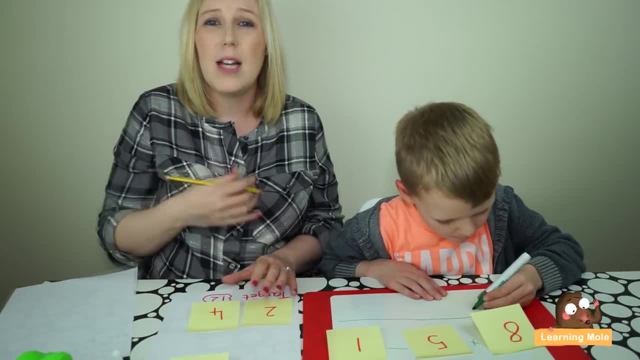 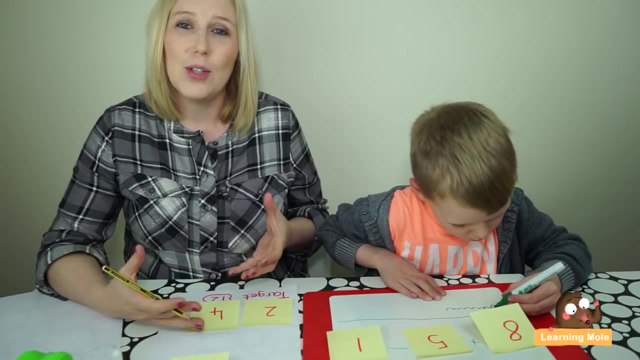 actually using little methods and strategies to work that out, and this, this is the value of this activity. you get all of that from just a simple bit of paper and a few post-it notes. you can use to make your target number as big or as little as you want, and also even if you want to use some